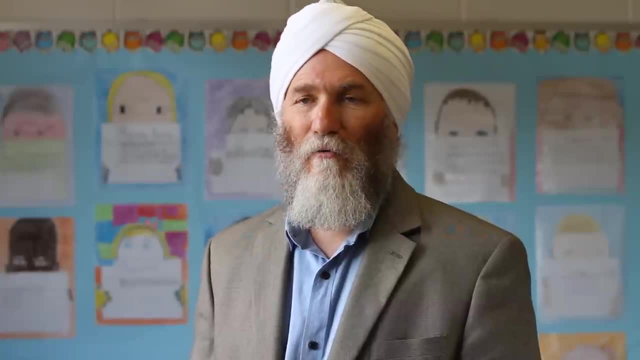 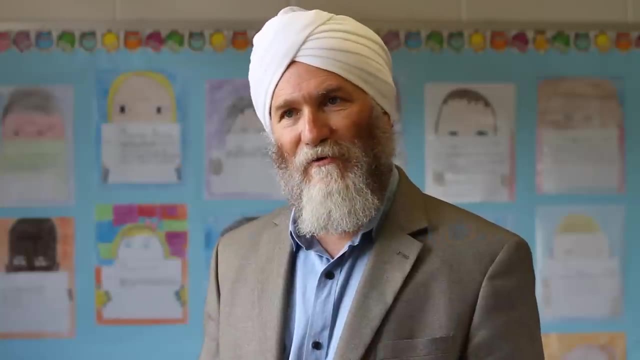 look like in an elementary classroom. We want people to see that. We want them to see the rich interactions, the clear learning trajectory that's taking place and the confidence in both students and teachers that's possible when things go the right way. All right do. 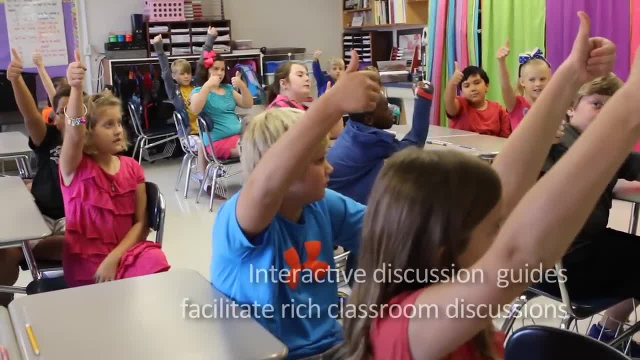 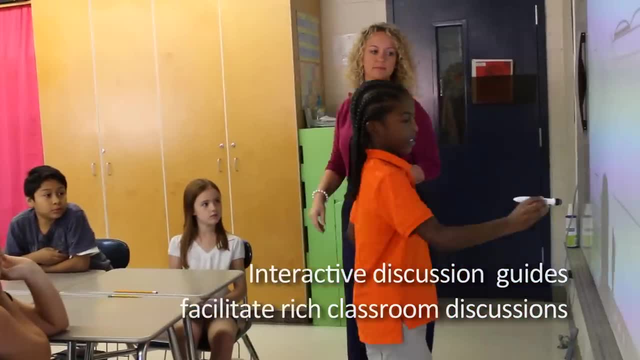 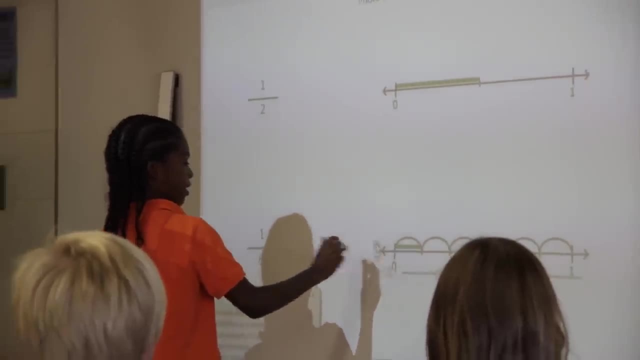 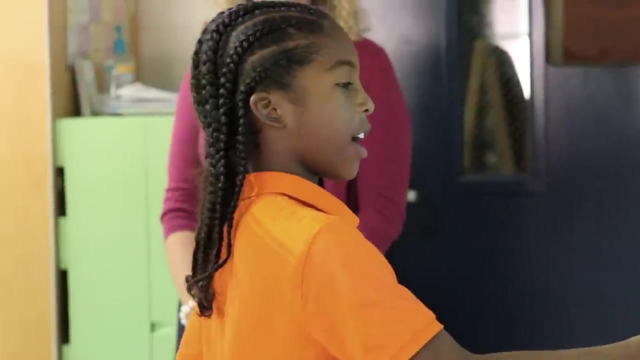 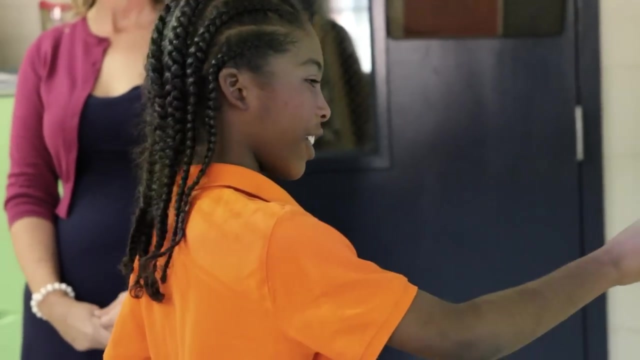 you agree with MJ? Thumbs up, thumbs down. All right, Damon, come show me how to build one sixth And explain to me what you did. I divide it into six pieces because the denominator is six and I shade it one because the numerator 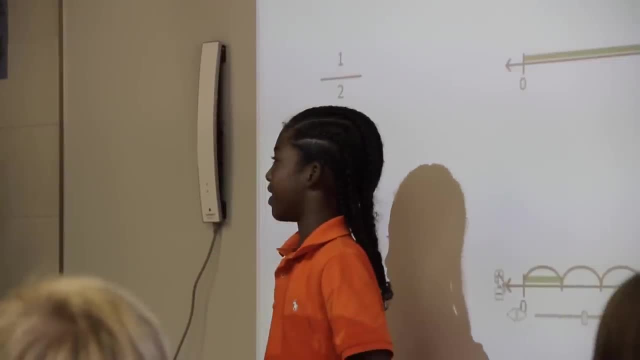 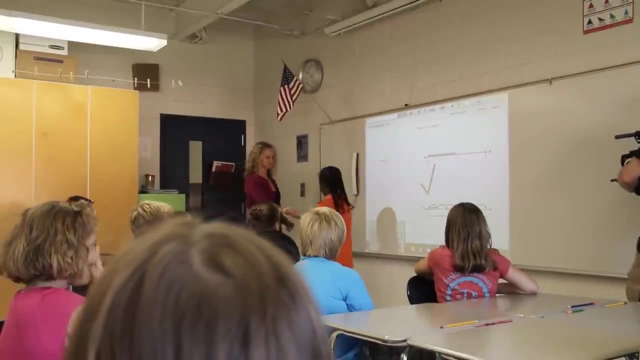 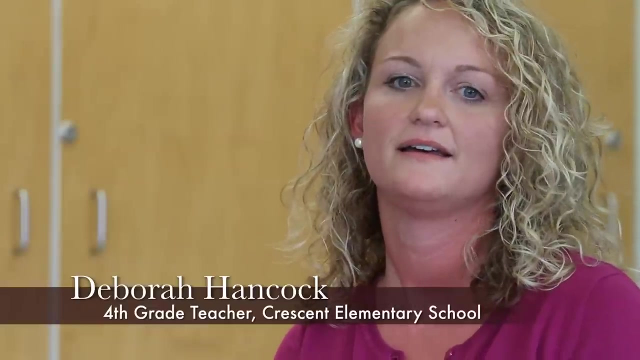 is one, and that's how many I shaded. Awesome job, And do we agree? Yes, All right, hit the check and check it. It initiates wonderful conversations in my classroom: seeing where my children are, knowing where they're at, hearing what they're going through, and 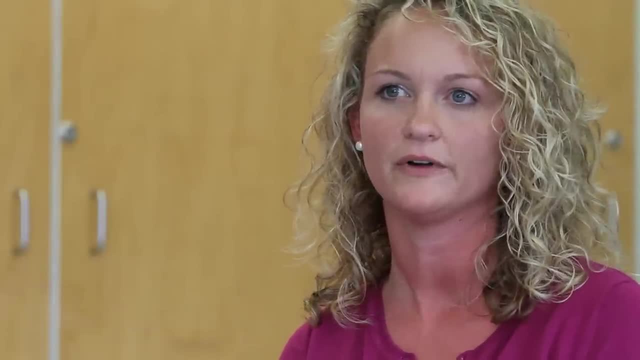 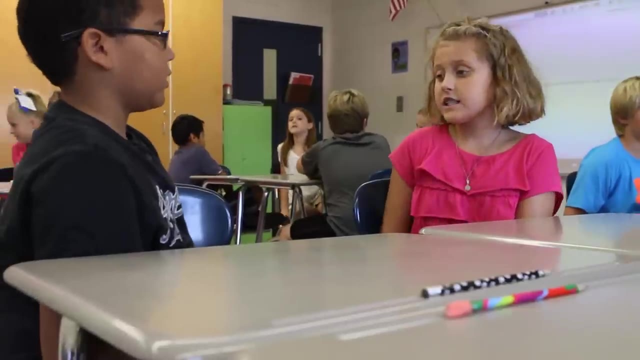 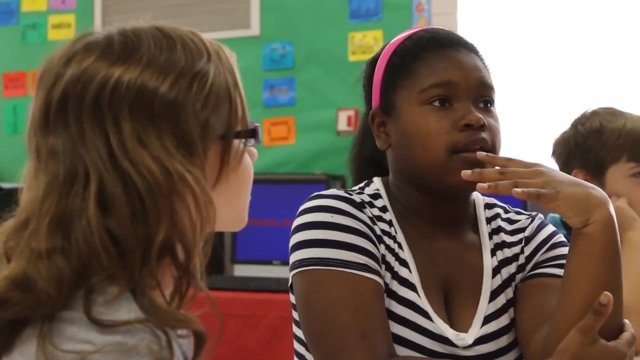 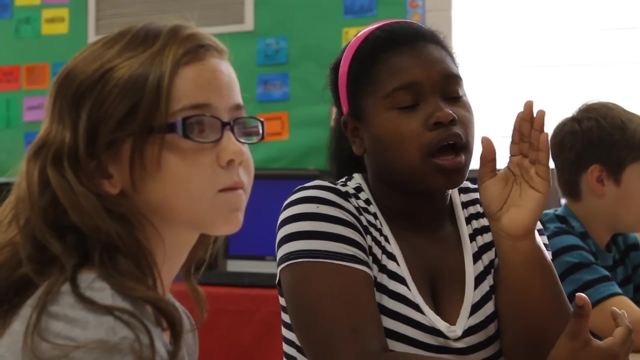 hearing them reason and justify and argue mathematically back and forth, seeing those moments when the light bulb goes off, knowing that they know it and that they could prove it to one another. That's what I love about Conceptual And wait. One sixth goes to close to zero and three sixths goes under the half, because 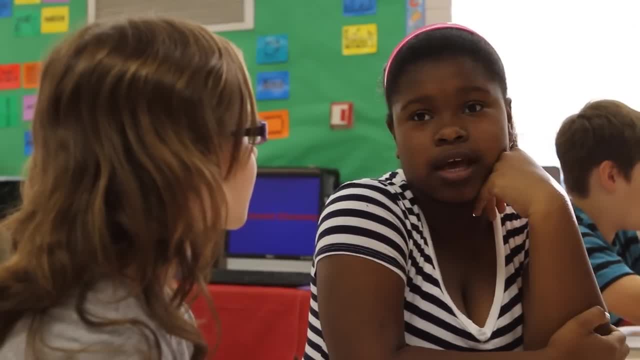 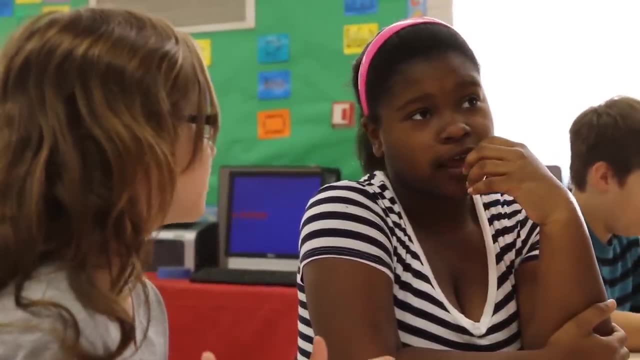 half of six is three and then five sixths goes close to whole, because it's almost half of six, Because if you draw it and I gave you color five in, it would be close to another six, So it would be close to a whole. 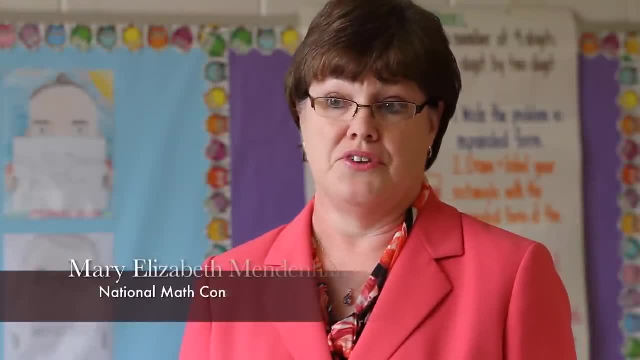 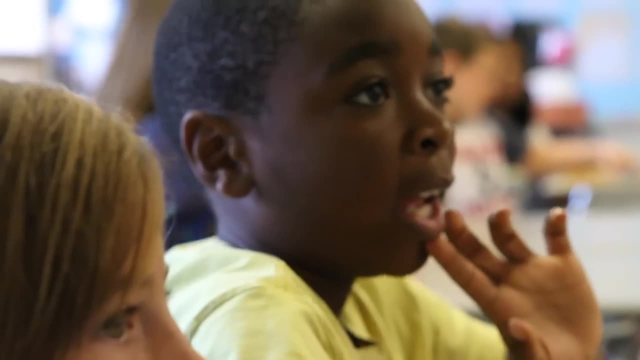 Classroom dialogue is the heart of knowing whether or not a student understands math or not. And if a teacher asks a question, we've got to hear the students talk about their thinking and reason about the math. And if we can have good discussions where children are making sense of the math rather than teachers telling to me that's a rich. 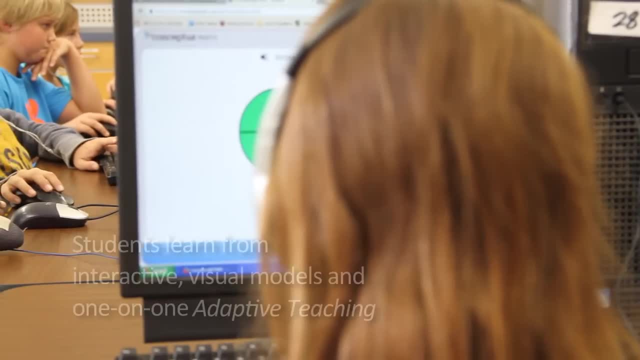 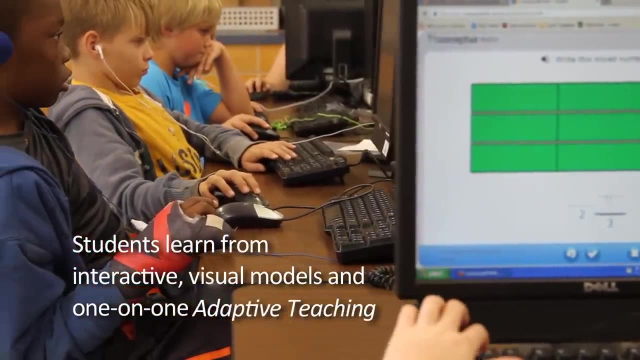 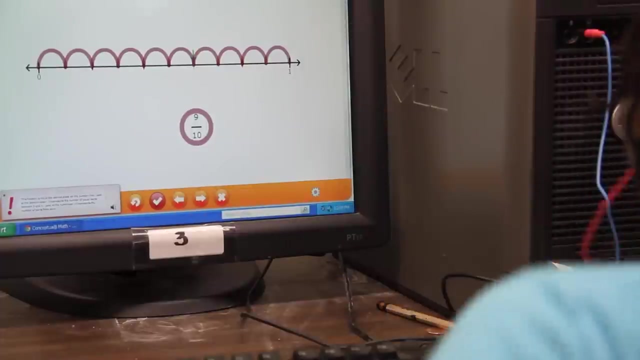 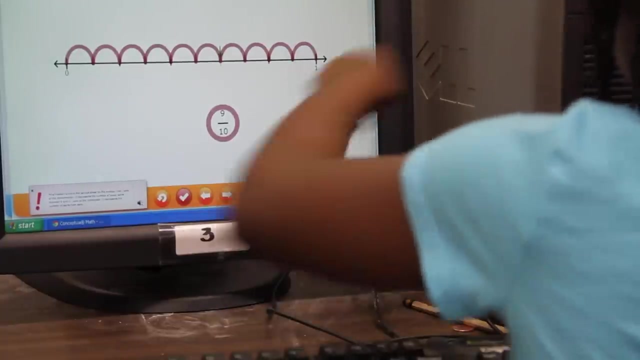 discussion. So if that is one whole, if that is zero and one whole, where would nine tenths be Right there? Would that be? if this is zero and this is one whole, where would nine tenths be Right there? 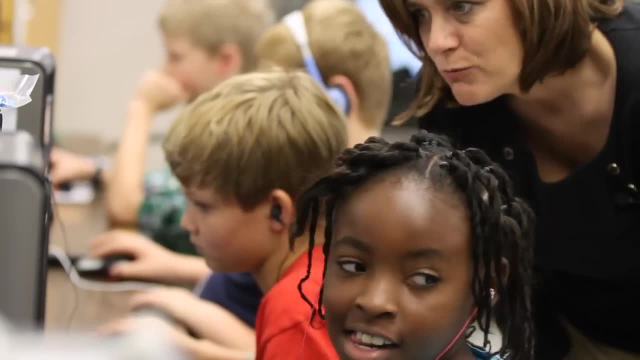 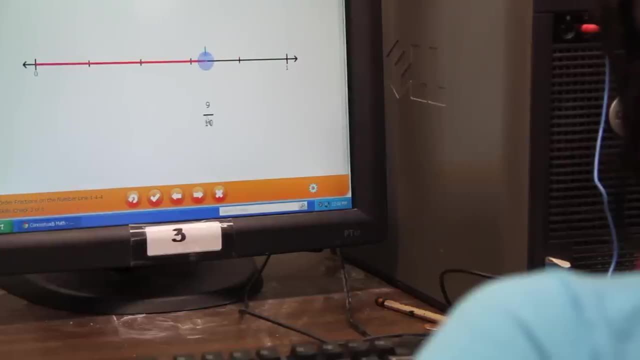 Okay, And how do you know? Because it's one less than a whole. It's one, what less than a whole? One equal part less than a whole. Okay, All right, Try that. Try it first. All right, let's talk about what we see on the screen. What was your score? 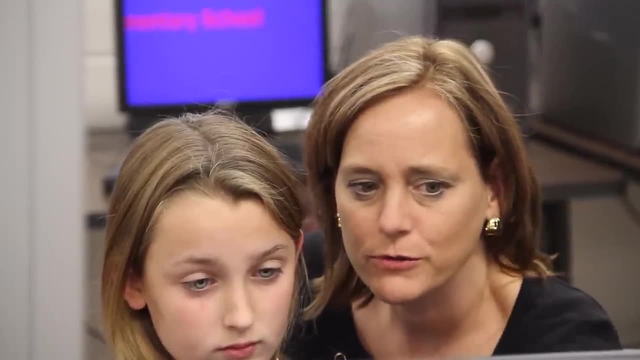 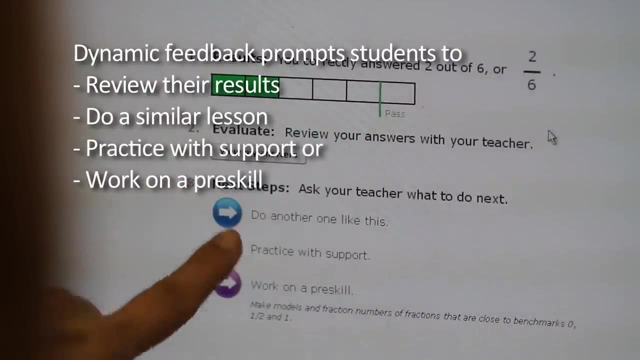 Two out of six. Two out of six, So we probably need to look at. we can review your answers and find out what you did wrong. Let's look at that first. Okay, so this one you missed. Why do you think you missed this one? 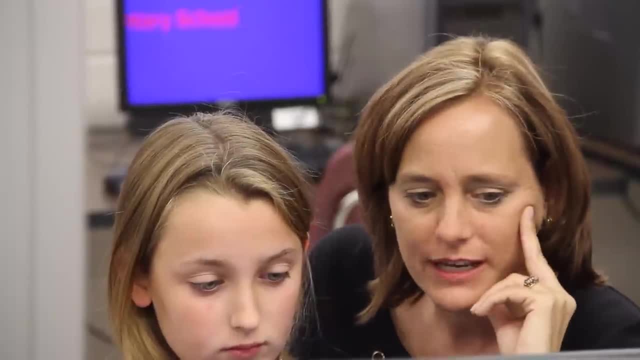 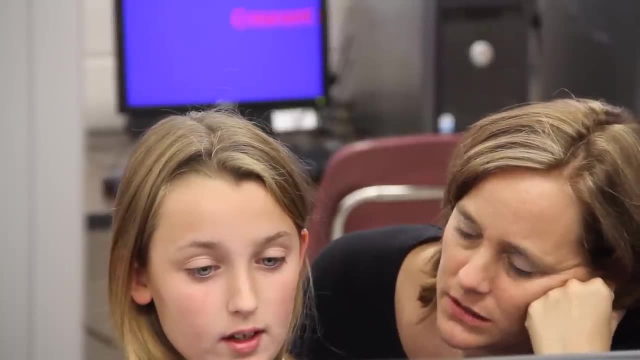 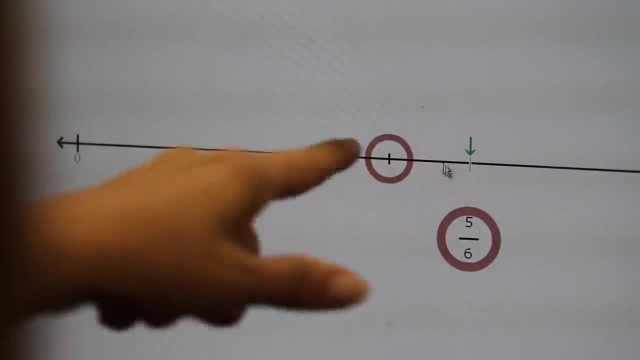 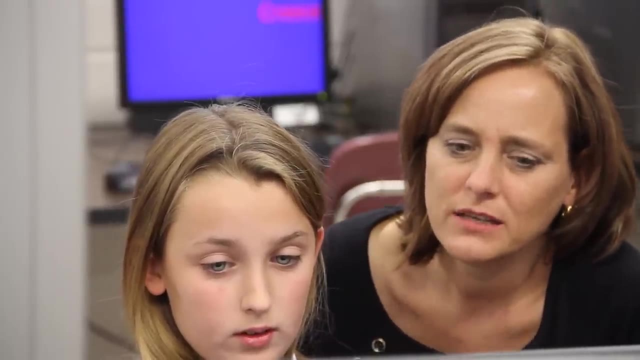 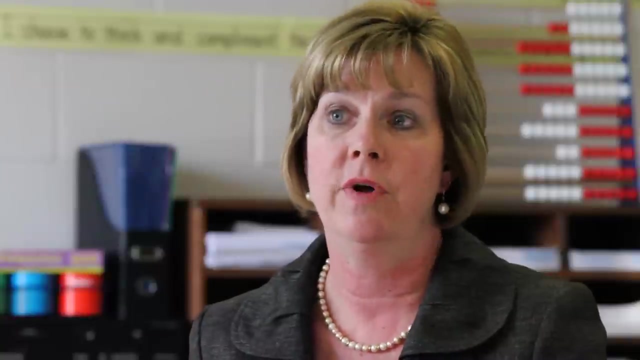 Okay, And so what? what is this benchmark? What's a half, And what is this benchmark- A whole? Okay, So what should five, six be Up here? Okay, I'm gonna try that. I think that CONCEPTUA has certainly changed the attitudes in a positive direction, for 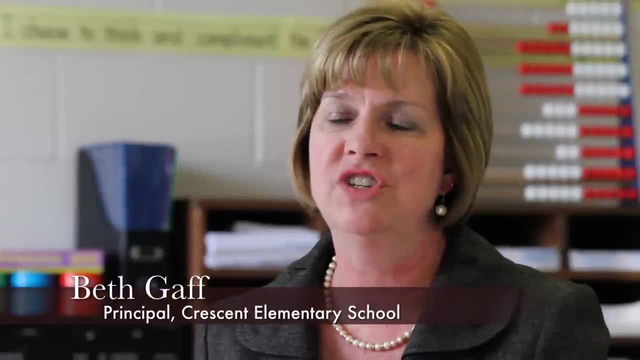 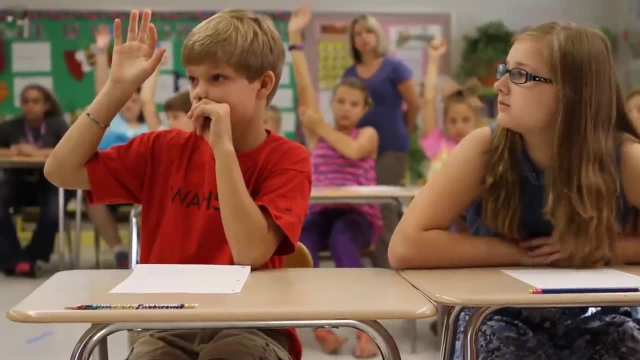 our students. When I come in and visit in our math classrooms, our students are confident. They know exactly what the teacher's asking them to do. If I'd come in a couple of years ago, they would be reluctant to share answers. 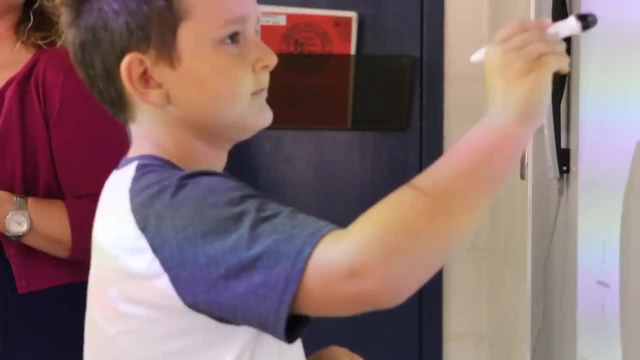 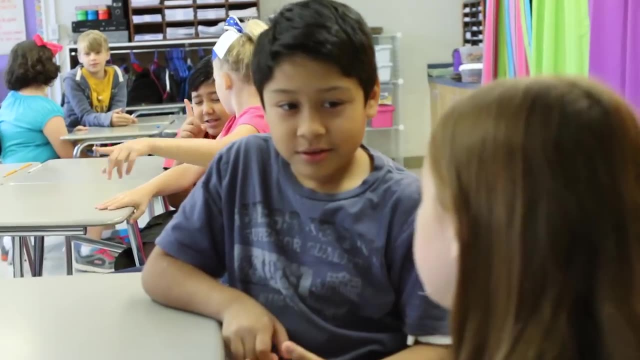 Now that's just a part of their math classrooms. They know that they're going to have to justify, They know they're going to have to explain why, you know whenever the teacher asks those questions. So that's just become an everyday part of what they do in their classrooms. 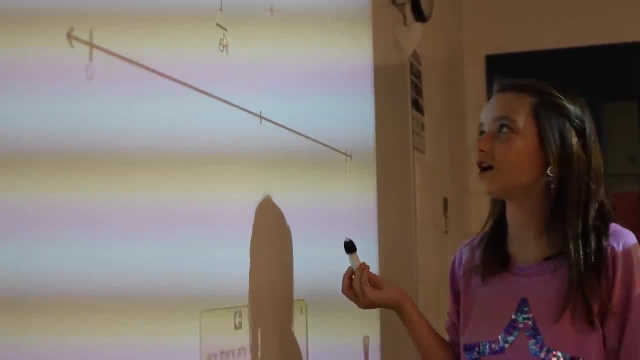 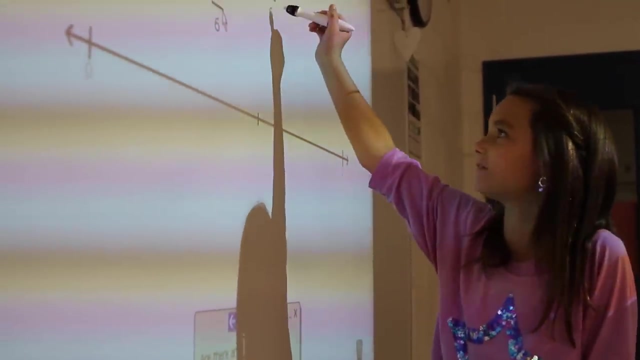 So I look at one-sixth and I automatically know that that is a unit fraction because the numerator is a one, And I know that one-sixth is the least out of three-sixths and five-sixths. so I know that I go somewhere around zero. So I put that right there And I look at five-sixths. 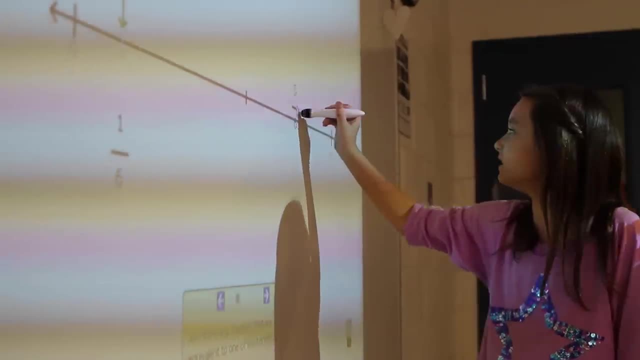 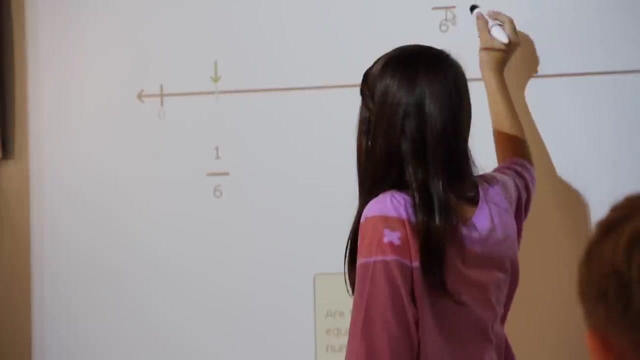 and I know that five is almost six, so I put it near the whole. And I look at three-sixths and I know that three is half of six, so I put it at the one-half mark. What do you think? Agree or disagree? Agree. 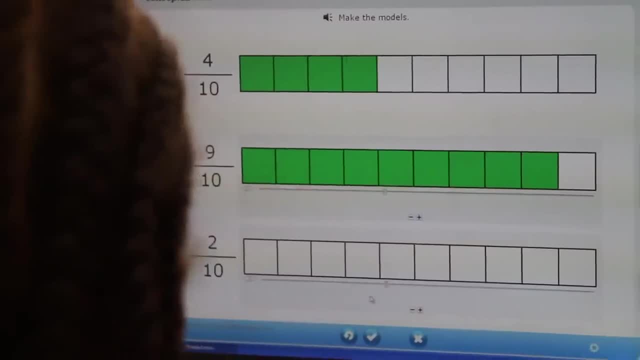 What can students do to help their students get a better understanding of math and math? What can students do to help their students get a better understanding of math and math? What conceptual does is give them the connections to the math learning. They need a visual so.